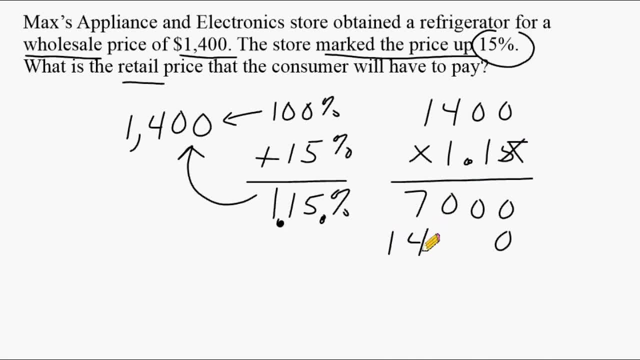 to hold this place And 1 times 1,400 is 1,400.. And now we have to put two zeros to hold two place values And, of course, 1 times 1,400 is 1,400.. And we add the columns up: 0,, 0,, 0,, 11.. 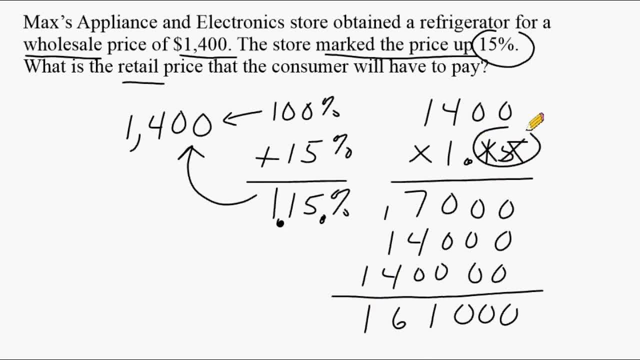 6 and 1.. And we have two numbers after our decimal, so we place it right here. So the retail price that a consumer will have to pay for this refrigerator will be $1,610.. Now another way that some people like to approach this problem is they just like to multiply. 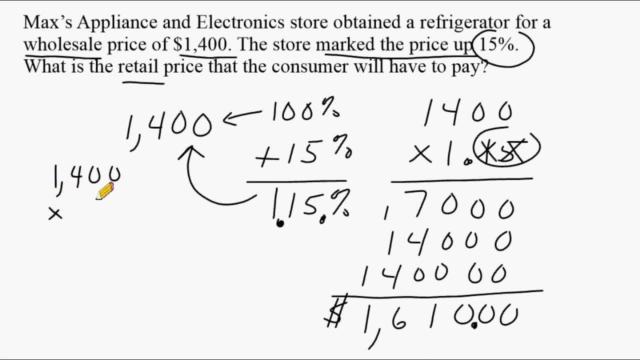 1,400 by 15%, but that will only show you how much the price increases by. That's not going to give you the retail price. So we're going to multiply 1,400 by 1,600. And we have to. 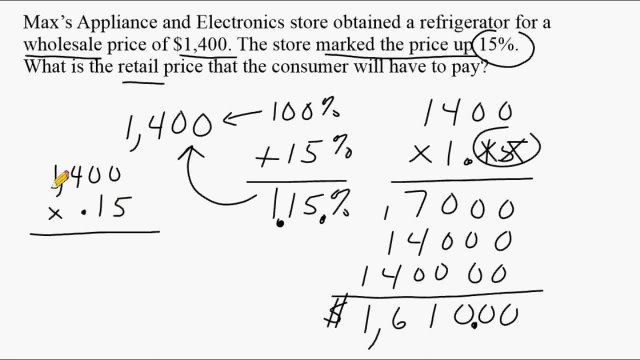 multiply 1,400 by 15%, but that will only show you how much the price increases by. That's not going to give you the retail price. That's just how much of an increase is there. So if we were to do that, let's see what we would end up getting. Alright, we write 1,400 here. That would be a. total of $210.. So some people just like to find the percent of the wholesale price and then they understand this is how much the price is going to increase by. But then you have to add that back to the original amount to find the retail price, And 1,400 plus $210 is $1,610. 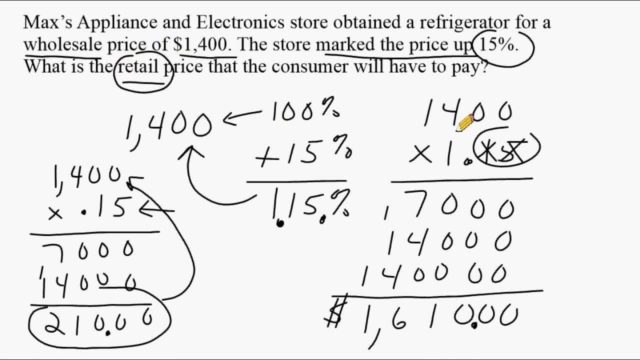 For me personally, though, whenever I find the retail price is something, I like to multiply the wholesale price by the percent increase added to 100%. So if the price increase is 15%, then I like to multiply by 115%, because you're paying 100% of the original amount plus a 15% extra. 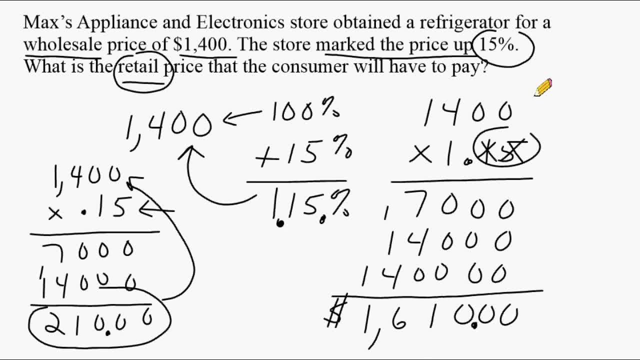 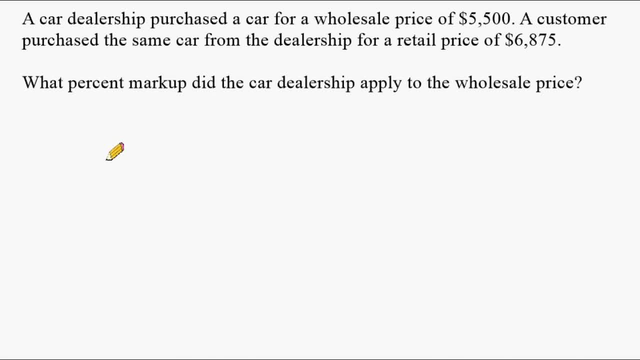 Alright, let's go ahead and do another example. Alright, this example is a little bit different than the previous example. In the first example, they gave us a wholesale price and then they gave us the percent markup. But with this example, they give us the wholesale price. 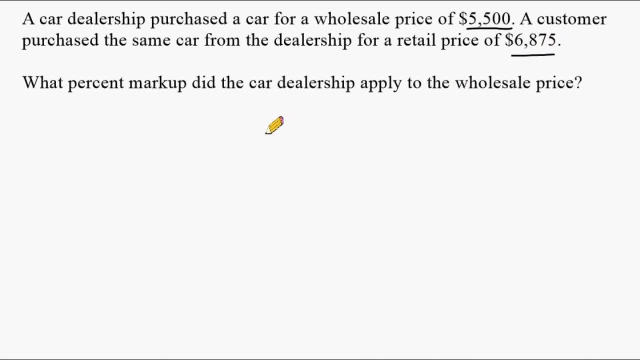 the retail price, and we have to use those two figures to determine the percent markup. So the first thing that we're going to do is we're going to take the retail price of $6,875, and subtract from that the wholesale price of $5,500. And what we see is that the price. increased by a total of $1,375.. So this amount right here represents a percent of the original amount. So what we have to do is determine what percent is $1,375 from the original amount of $5,500. And that's going to be the percent markup that was applied. to $5,500.. Alright, so what we have to do next is we have to take $1,375 and divide that by $5,500. And that is going to give us a decimal value, and then we have to take that decimal. 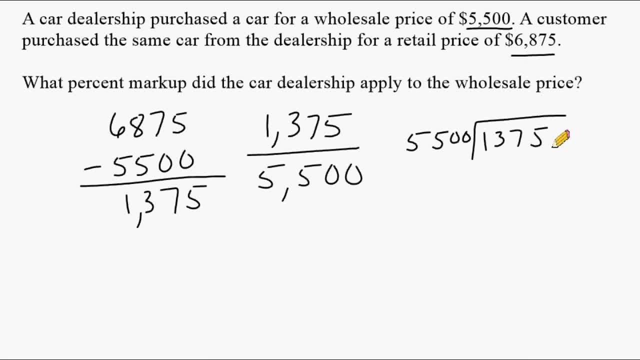 amount and convert it into a percentage. So what we have to do, since this number on the inside is smaller than this outside number, is we have to add a decimal here, here, and we add a zero in the first place value, after the decimal, which is the tenths place. 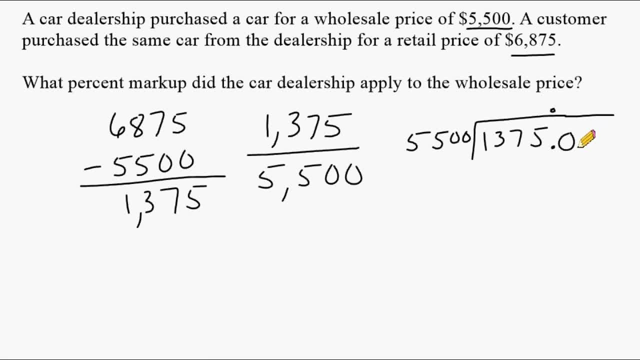 And then we continue to add zeros if needed. Alright, so what we're going to do is divide $5,500 into $13,750.. So we know that 5,000 times 2 is 10,000, and times 3 is 15,000,. 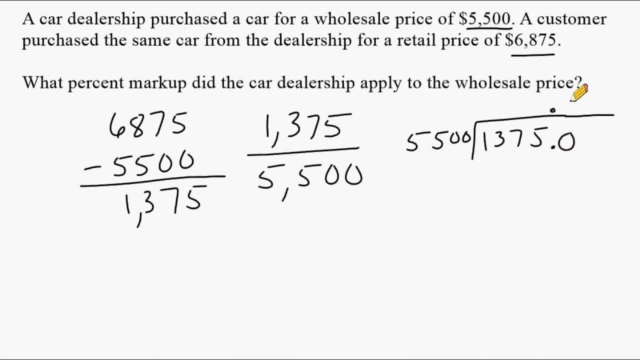 and that would be too big. So this only fits into here two times. And doubling $5,500 is $11,000. So we subtract $11,000 from $13,750, which gives us $2,750.. Now we add a zero in the next place value and drop it down, And I'm going to estimate. 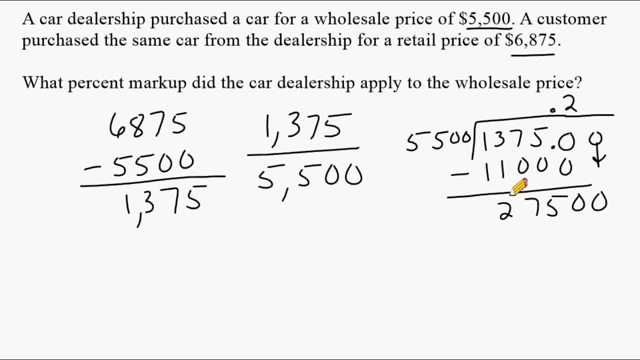 here. this is about $5,000, and this is a little bit over $25,000. And I know $5,000 goes into $25,000 five times. So if we multiply 5,500 by 5, we end up getting exactly $27,500.. So this fits into here exactly five times. 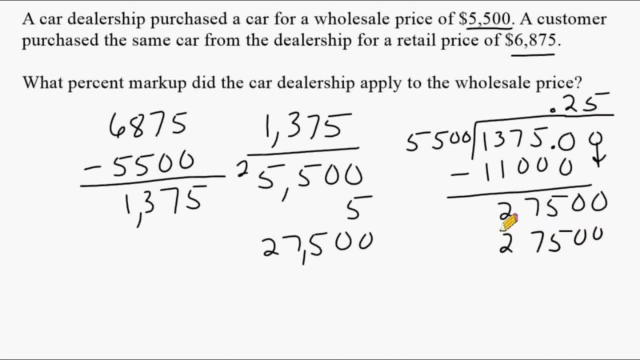 leaving us with no remainder. So to convert this into a percentage, we just take the decimal point and move it two spaces to the right. So we would say that the car dealership marked up the wholesale price by 25%, which means the consumer is going to pay 125% of the wholesale price. 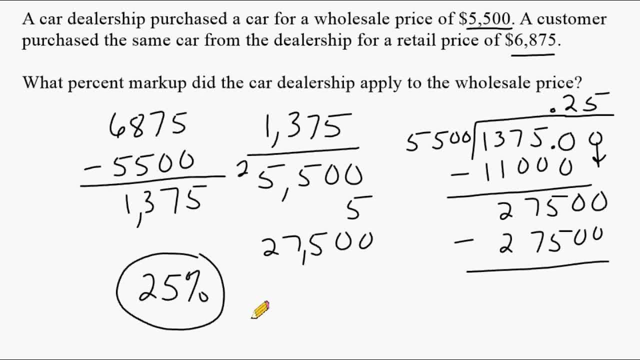 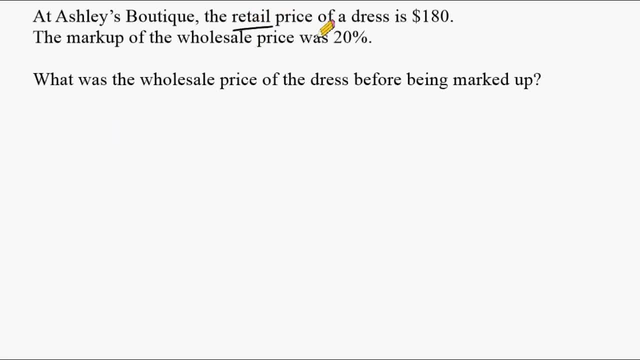 All right, let's do another example. All right, this problem reads that at Ashley's Boutique, the retail price of a dress is $180.. The markup of the wholesale price was 20%. What was the wholesale price of the dress before being marked up? 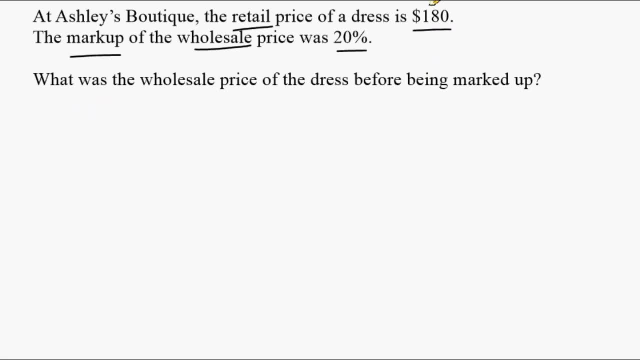 All right. so they give us what the price is going to be that the consumer will have to pay, or the retail price, and they give us what the markup was. So we have to work backwards to figure out what was the price that the boutique obtained the dress for. 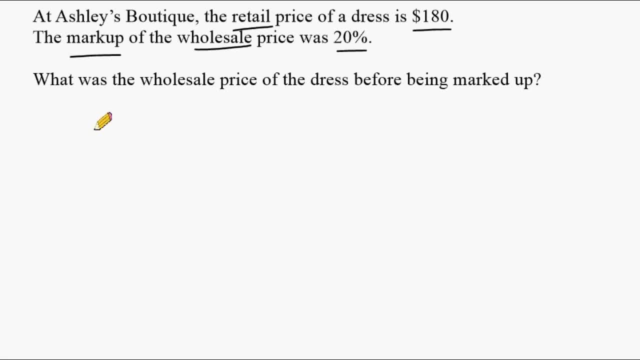 What was the wholesale price of that dress? So in general, what we've been doing is we've been starting with the wholesale price and then we've been multiplying that by the percent markup added to 100%. So we've been taking 100% and adding that to whatever the markup price is. I'm going 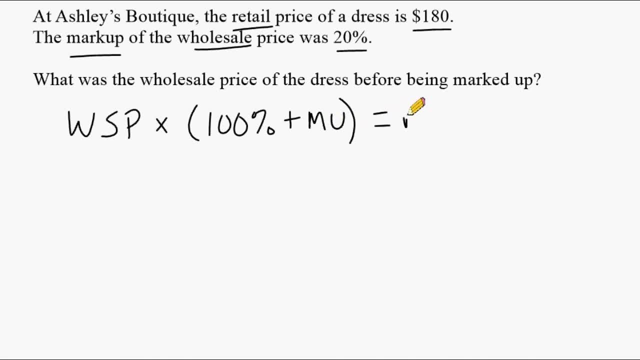 to put MU for markup, and that's going to be equal to the retail price. So what we're going to do here is this: They don't give us what the wholesale price is. so what I'm going to do is I'm just going to put a W for next. 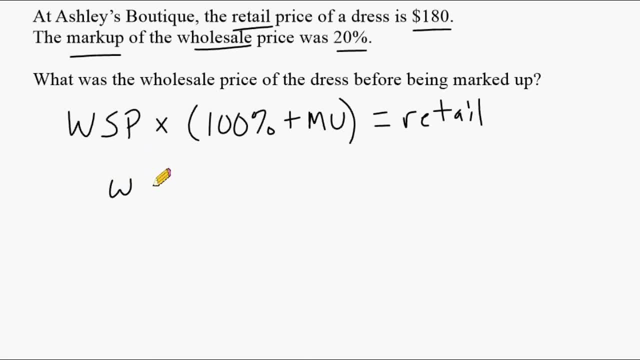 So what I'm going to do is I'm going to put the wholesale price And then I'm going to put a W for the retail price, which is $20.. So what we're going to do is we're going to take the wholesale price and we're going 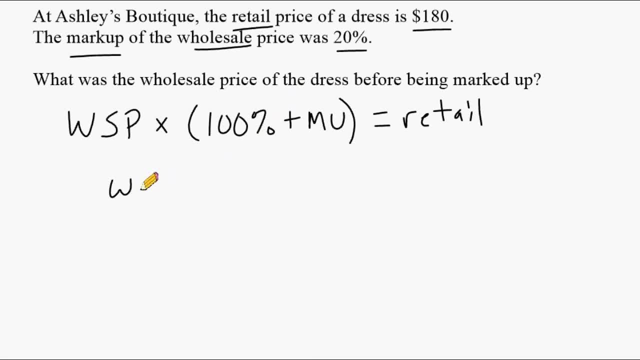 to add that to that W. I'm going to add that to $20. And that's going to give us what it's going to be. So we're going to add that to $20. And we're going to put that to our wholesale price and we're going to multiply that by. 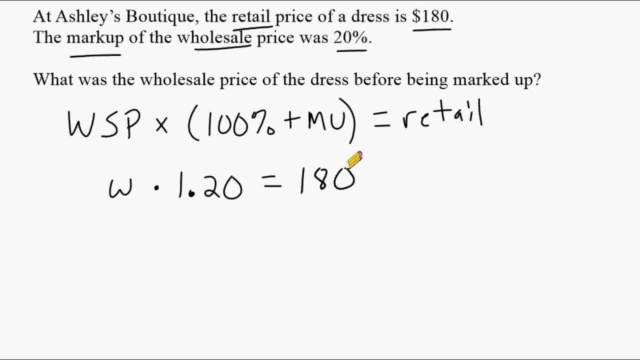 120%, And that's going to be equal to the retail price which is given, and that is $180.. Now, if you notice, here, what we have is really an L2. algebraic equation in a quite simple one. So I can switch these out because of the 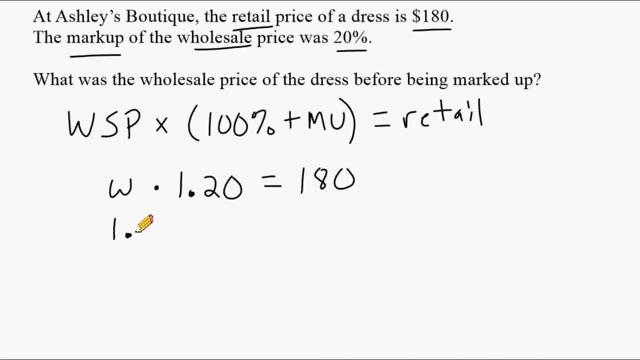 commutative property of multiplication. I'm going to simplify 1.20 to be 1.2 and just write a w after it equals 180.. And all we have to do now is solve for w. And the opposite of multiplying w by 1.2 is to divide by 1.2.. So all we 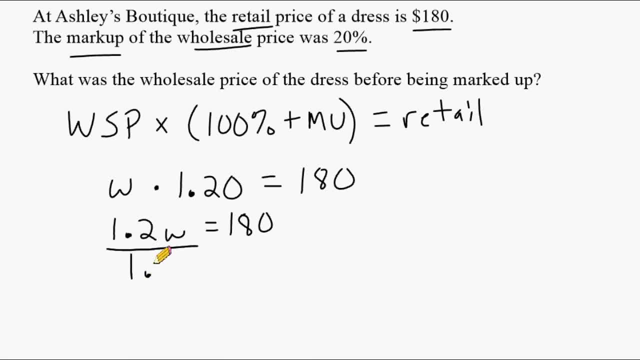 have to do is divide this side by 1.2, so 1.2 cancels with itself. It doesn't cancel out to nothing, It's really just 1.. So we write 1w at the bottom And on the right. 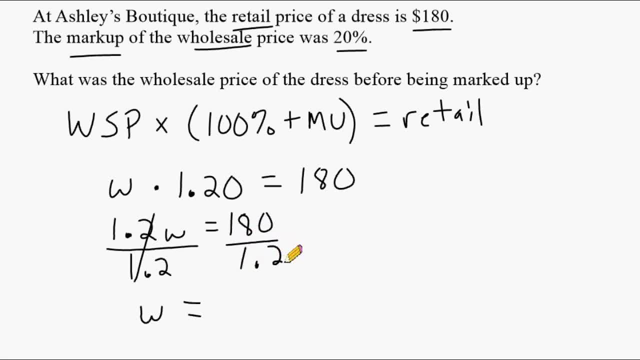 here we divide 180 by 1.2.. So let's go to the side here and take 180 and divide it by 1.2.. Alright, because we have a decimal in the divisor, we have to write one in the dividend And we have to move this.